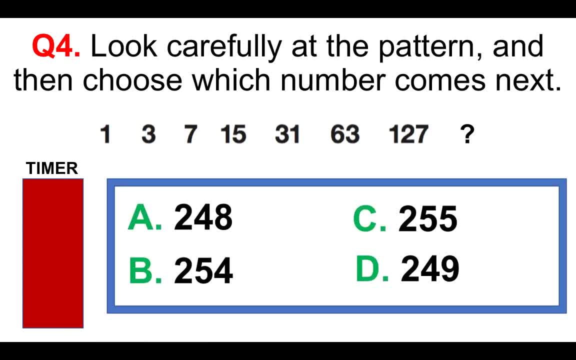 which number comes next? Is it A 248.. B 254. C 255. Or D 249.. If you get this one, you're a genius. Don't forget to put your answer in the comments section below to question. 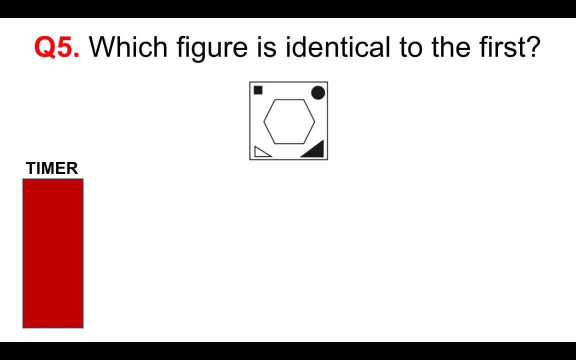 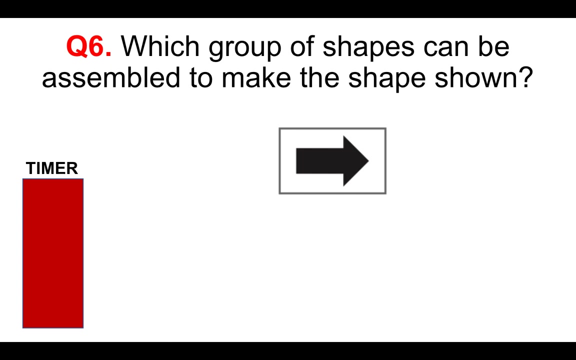 four and the others: Okay, Question number five: Which figure is identical to the one that's shown? Is it A, B, C or D? Okay, Question number six. Which group of shapes can be assembled to make the shape that's shown here? Is it A, B, C or? 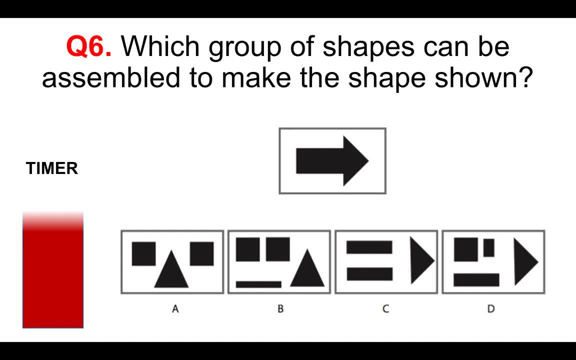 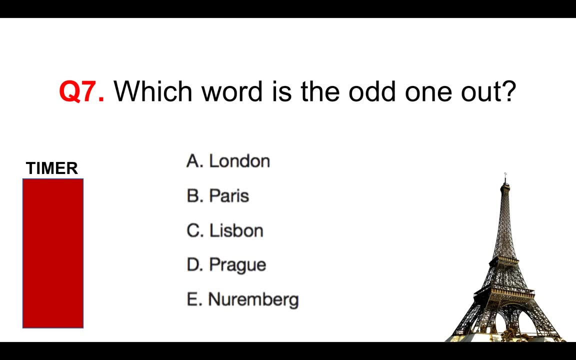 D. Moving on to question number seven. now, Which word is the odd one out? Is it A- London, B, Paris, C, Lisbon, D, Prague or E Nuremberg? Which word is the odd one out? 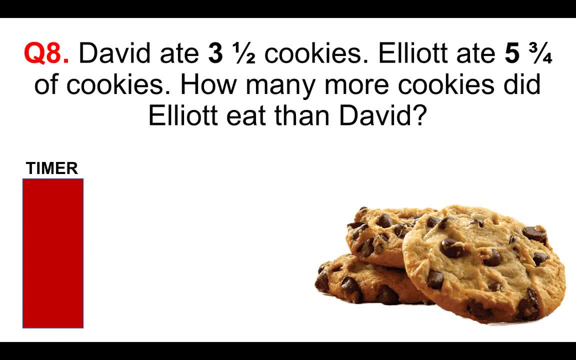 Moving on to question number eight, David ate three and a half cookies. Elliot ate five and three quarter cookies. How many more cookies did Elliot eat than David? A, Two and a quarter, B, Two and a half, C, Three or D, One and three quarters. Again, please. 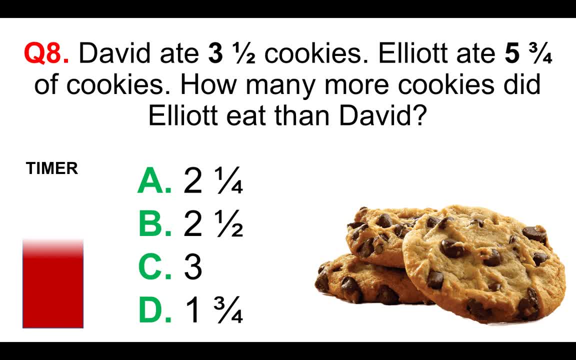 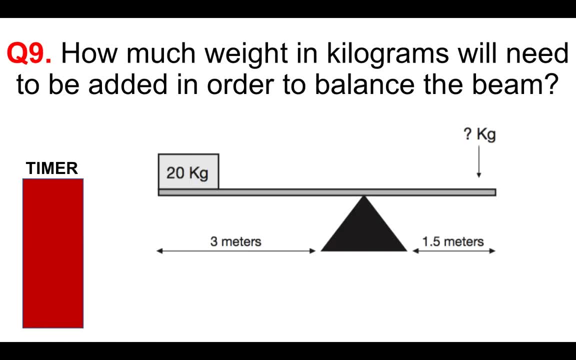 put your answer in the comments section below. Moving on to question number nine, How much weight in kilograms will need to be added in order to balance the beam? A- Ten kilograms, B- Twenty kilograms, C- Thirty kilograms Or D- Forty kilograms? Quite a difficult question. 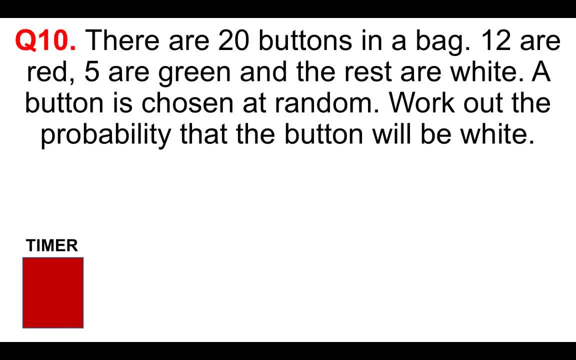 Question number ten. There are twenty buttons in a bag. Twelve are red, five are green and the rest are white. A button is chosen at random. Work out the probability that the button will be white: A- Three twentieths, One out of ten. B- Twenty kilograms. C- Thirty. 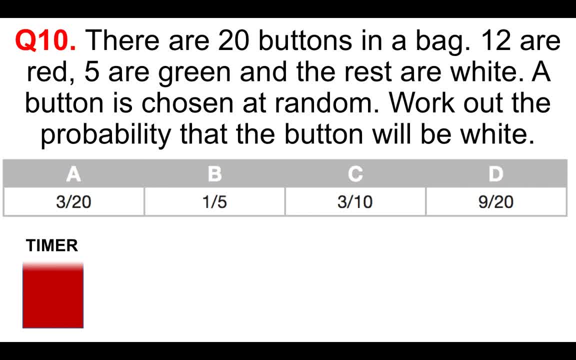 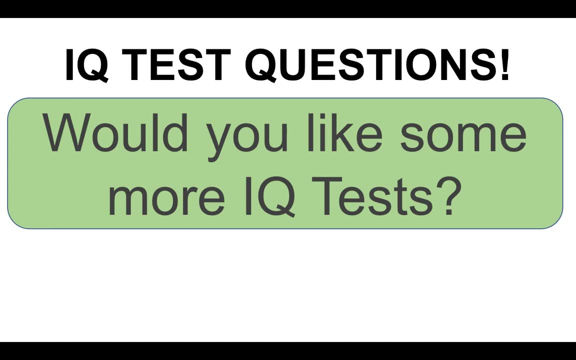 out of five, D Three out of ten Or D Nine out of twenty. Okay, guys, don't forget to put all of your answers in the comments section below and I'll come and mark them. Let me know what you thought about the test. If you'd like more,